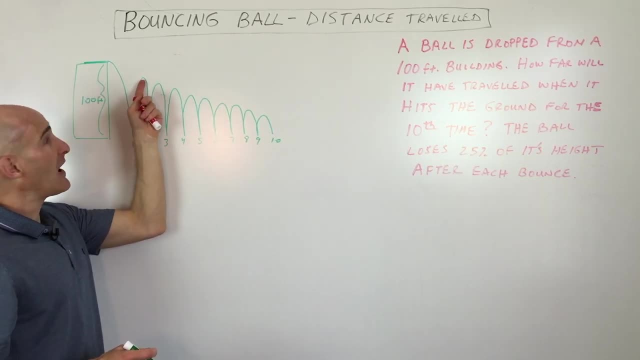 you drop it the first time, that's 100, then it's only going up 75 feet, but it's also traveling down 75 feet as well. So what we're going to do is we're going to look at a few of these terms in. 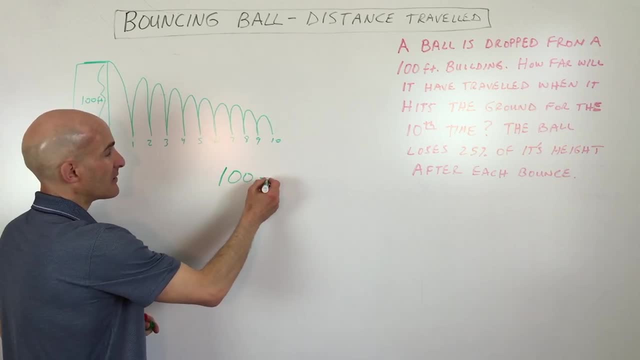 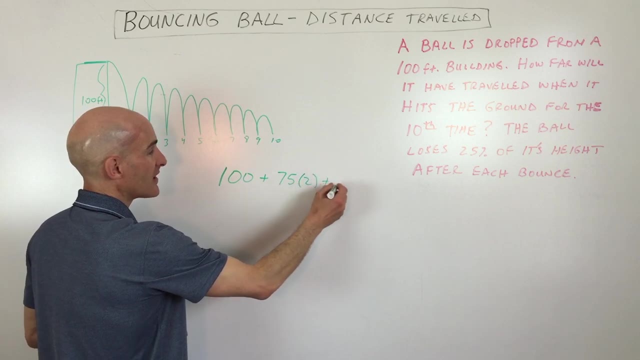 the sequence. So the first term is 100, right, Okay. then the next term is going to be 75. Okay, and then the next term after that. of course, you're going to have two of these, right? The? 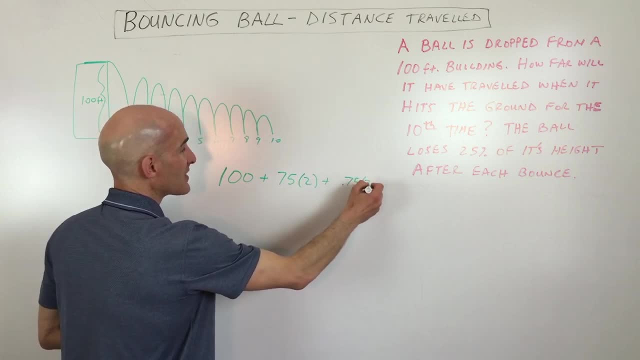 next term after that is going to be 75% of 75. And then the next term of that is going to be 75% of that And because it's losing 25%, it's retaining 75% of its height. So the way I recommend doing this problem is: 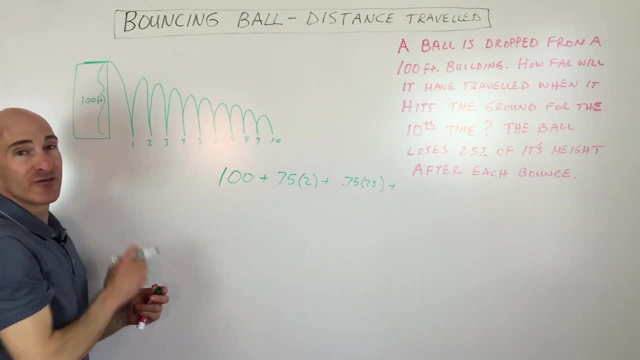 let's ignore the 100 feet when it initially falls, Okay, let's just work with these ones where it's going up and down, And what we're going to do is we're going to treat it as a geometric sequence, Okay, and we're going to add up all those terms in the sequence that makes it. 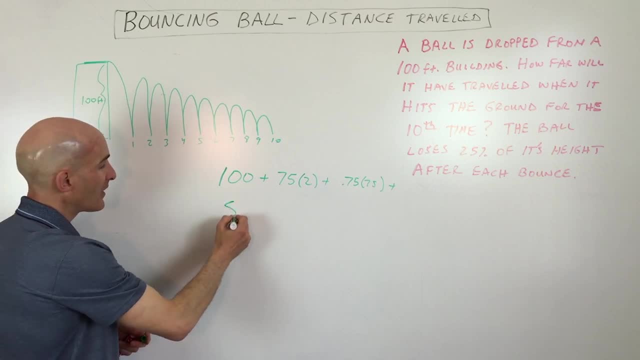 a series, And the way we're going to do this is we're going to use the formula: equals a sub one, one minus r, to the n all divided by one minus r. So this is the formula you want to use when it's a finite geometric series. r is the ratio. Okay, that's what you're. 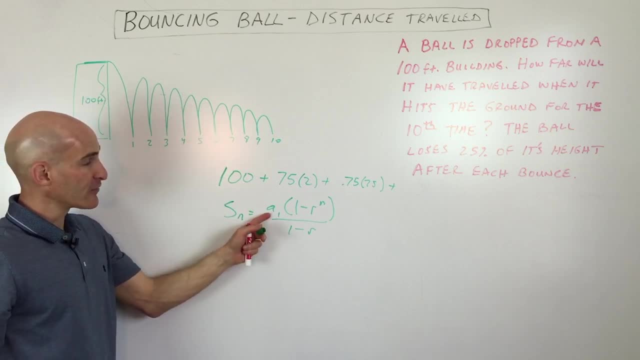 multiplying by each time, That's 75%, Okay. And then the first term is a sub one. And again this r is also the ratio, what you're multiplying by to get to the next term, and n is the number of terms. So what we're going to do is: the first time it bounces up here, that's going to be our. 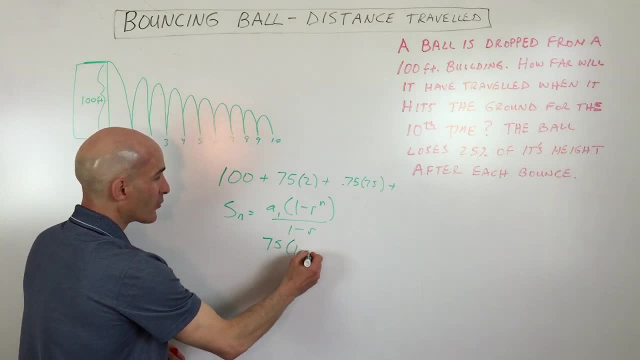 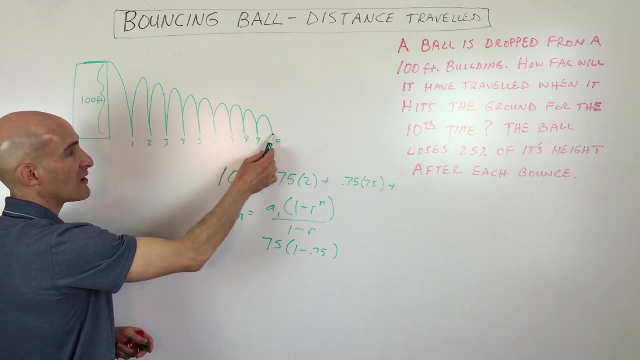 first term, we're going to treat that as 75 feet. The ratio is 0.75.. And then what happens is, you can see it's going to go up and down, Okay, even though when it hits that ground for the 10th time it's not continuing. So there's going to be. 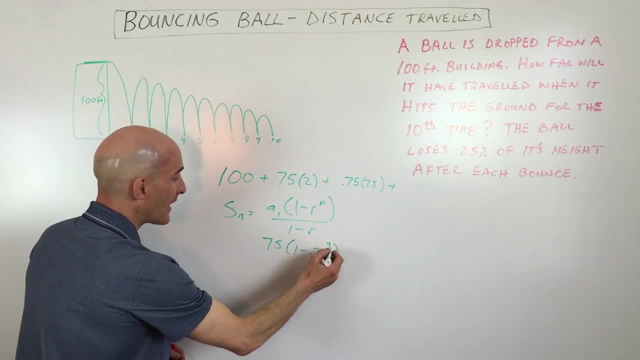 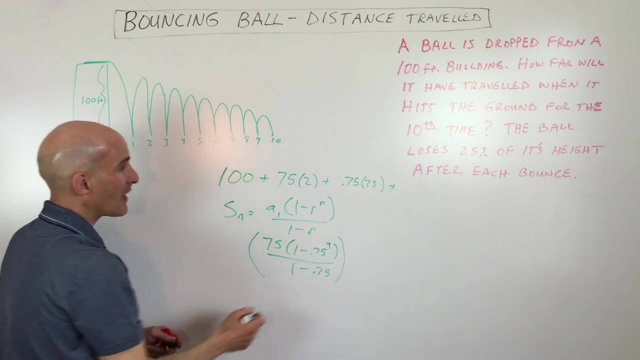 nine terms from here to here, So n is going to be nine all divided by one minus 0.75.. And then what we're going to do is we're going to take that and we're going to double it because we want to. 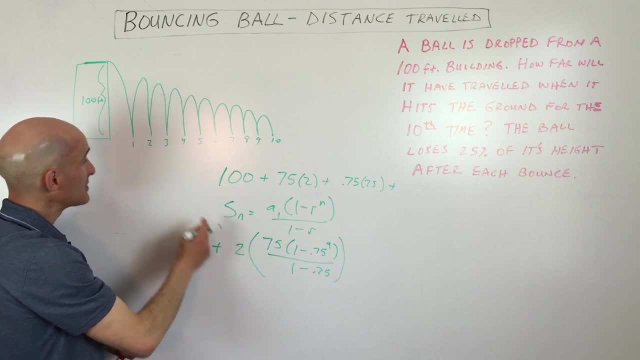 count the up and down, So that's going to be times two, Plus we're going to add that initial drop and so that's going to be 100. So this will give us the total distance traveled, And I hope that makes sense to you. If not, go ahead and take a look at the video again. It's just a geometric.